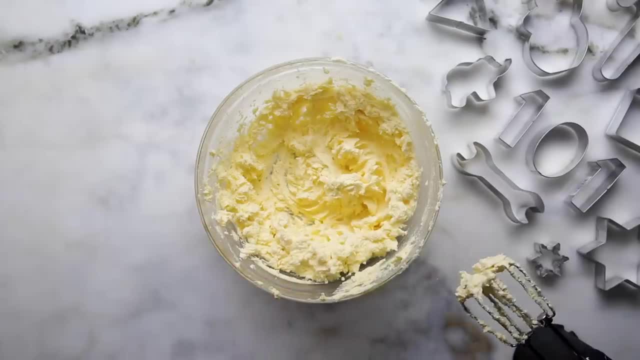 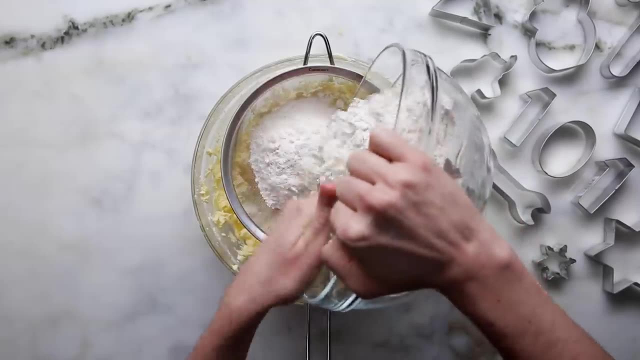 and sugar. So once we have the liquids well incorporated, we're going to add a little bit of kosher salt here Again, not to make it salty, just to be a flavor enhancer and balance out that sweetness. And so now we've got that in there, We're going to add our all-purpose flour And 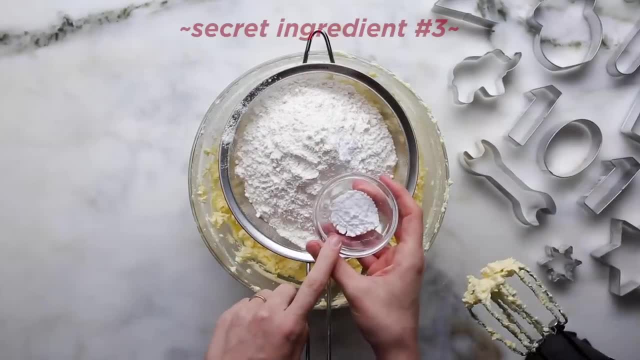 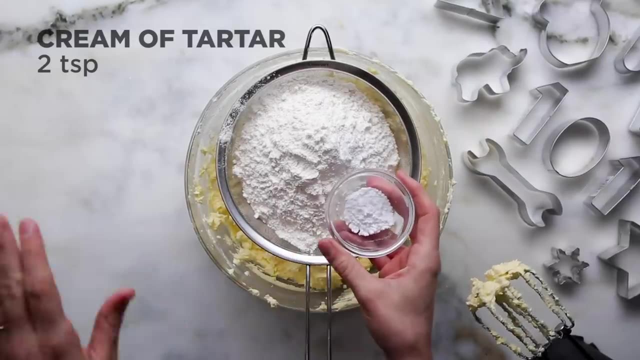 next goes in a little bit of baking powder, And this ingredient is our third little secret ingredient for this recipe: cream of tartar. Cream of tartar is actually what's left over in the barrel wine making And it's basically like just an acidic ingredient. So you're adding this and this. 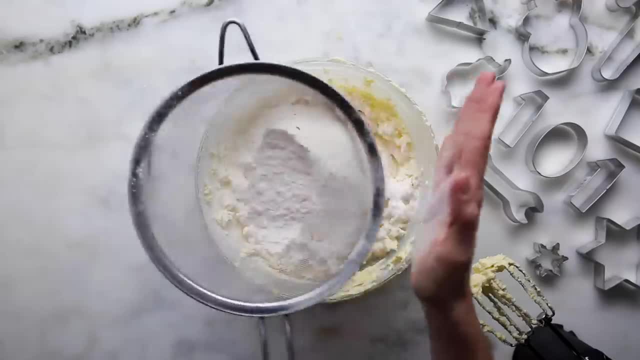 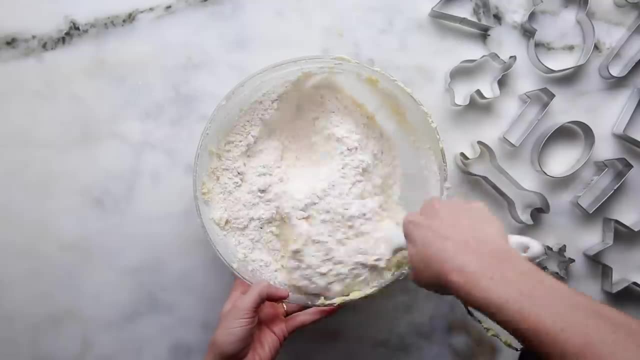 is going to help with a few things. It's going to give us like a really cool texture in the end, And it's also going to prevent the cookies from browning too much. So I'm going to fold in just to get it started, because there's a lot of flour in here. I don't want to make a huge mess, So I'm 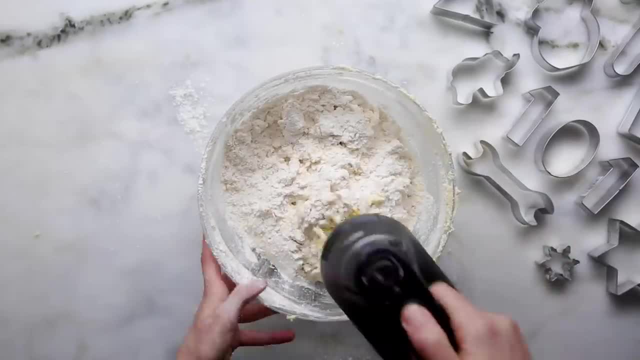 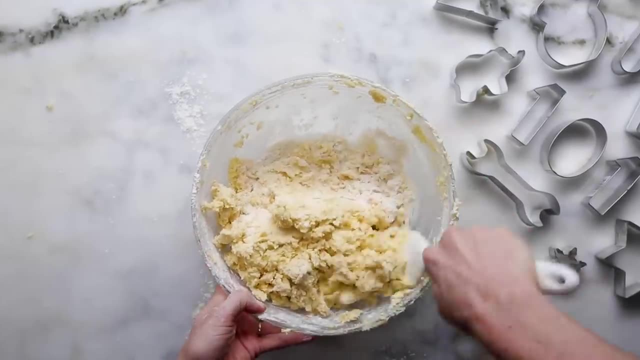 going to fold to get it started, finish incorporating it with the beaters because it is a pretty dense mixture. There's a little bit of floury bits that aren't fully incorporated. That's fine Again to have like a really flaky and snappy cookie. you just want to fold it in You. 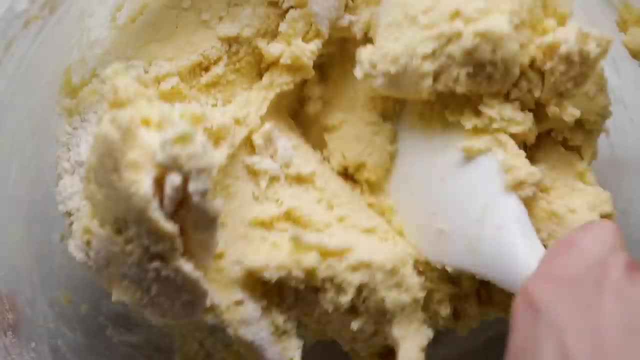 don't want to make a mess, So I'm going to fold it in. You don't want to make a mess, So I'm going to fold it in You and snappy cookie. you don't want to overwork this mixture, So you're kind of like just. 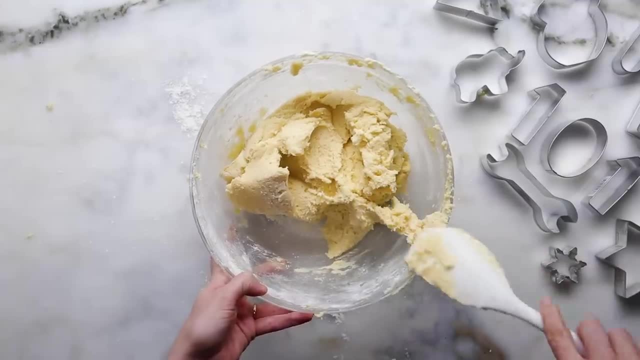 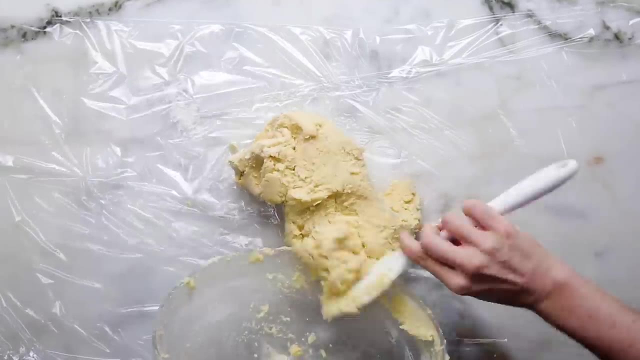 incorporating the flour. You don't want to go much more than that. This dough is almost kind of similar to like a pastry, where you want to keep it cold all the time. There's a lot of butter in here, So if it gets too greasy it's going to be really, really hard to work with, And you're not. 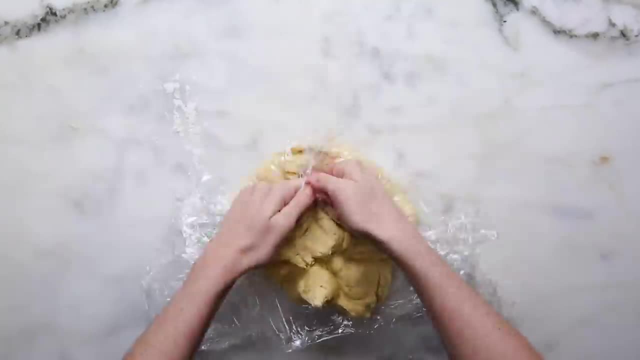 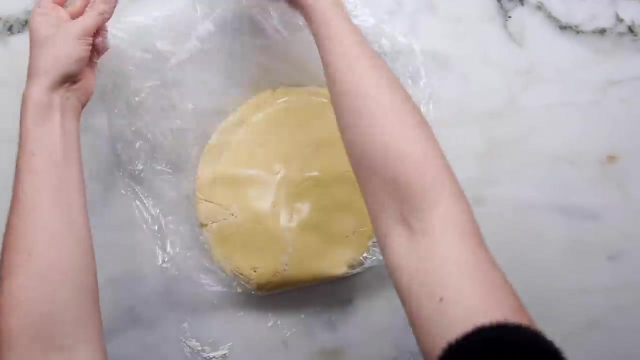 going to have really clear, defined shapes. Dough goes on in some cling film And then you can use the cling film to kind of like pull the pieces together. It's just like kind of sticky. So this is a really easy way to not make a huge mess. So this is going to go into the fridge And then we 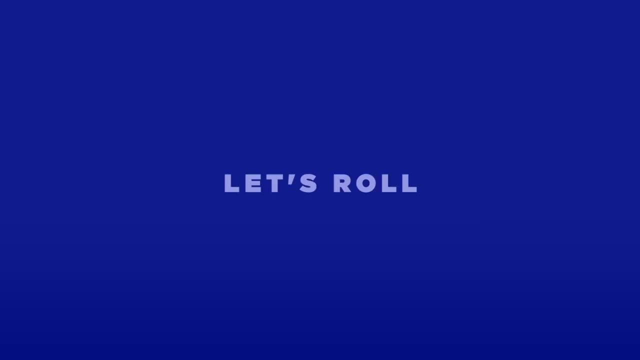 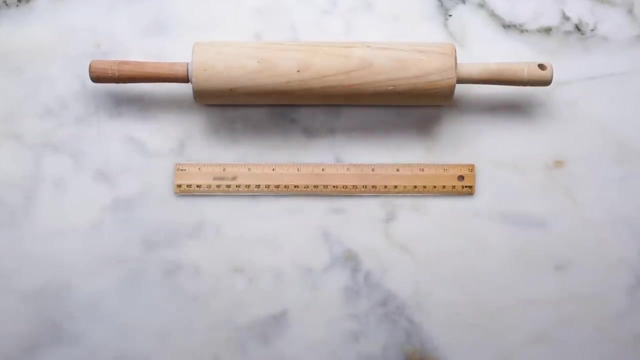 will roll it out in about two hours. Here are a few things you might need for rolling out your cookies. You need a rolling pin or a wine bottle, whatever you have at your house- And then something to measure the thickness with a ruler. or our fourth little trick of this video, which we'll get. 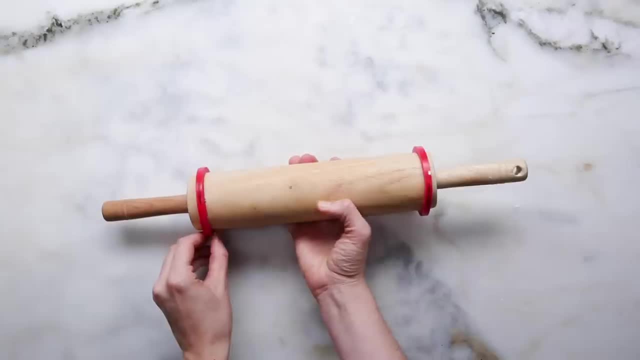 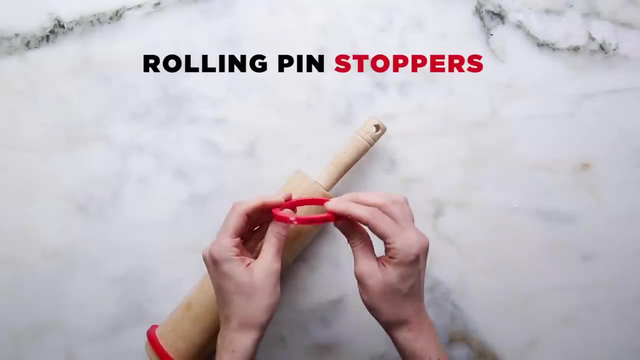 to later, If you are making a lot of cookies or you're like an avid baker. they do have these like kind of cool rubber rolling pin thingies- I don't know what you call them- like a rolling pin, stoppers, guards. maybe it really makes sure that you get like that perfect quarter inch, But you have to. 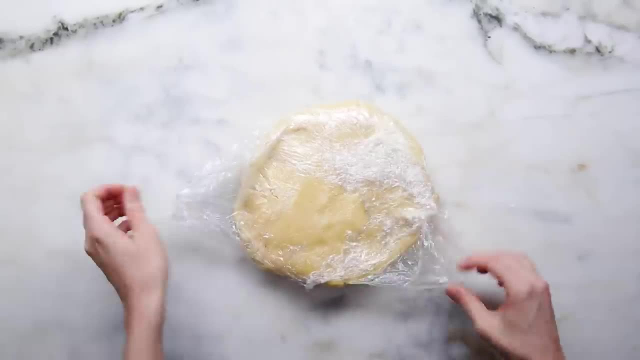 have like the perfect size So you can roll it out in about two hours. And then you can roll it out in about two hours, But you have to have like the perfect size rolling pins and you have to buy them their specialty. So we're going to show you a hack. So the enemy of rolling out anything is 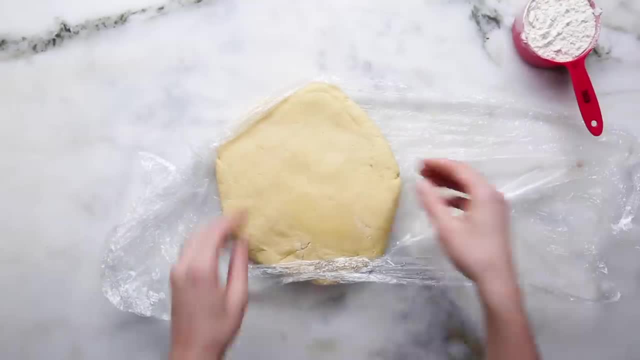 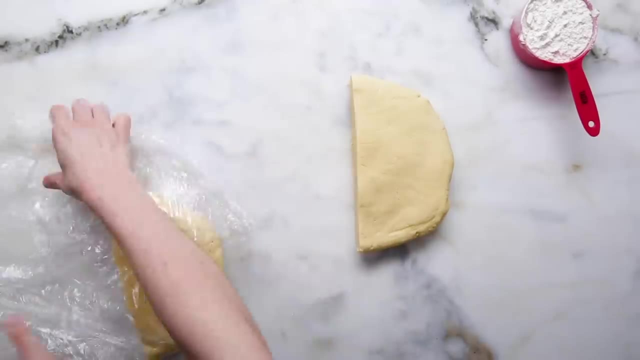 sticking to the surface that you're working on, So have a little bit of flour nearby. As you remember, we want to keep our dough super cold, So I'm going to work in batches. I'm going to put half of this back in the fridge and only roll out half at a time. Alright, so this is the trick that we learned. 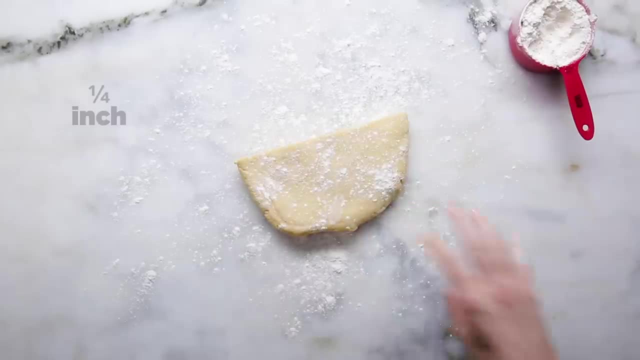 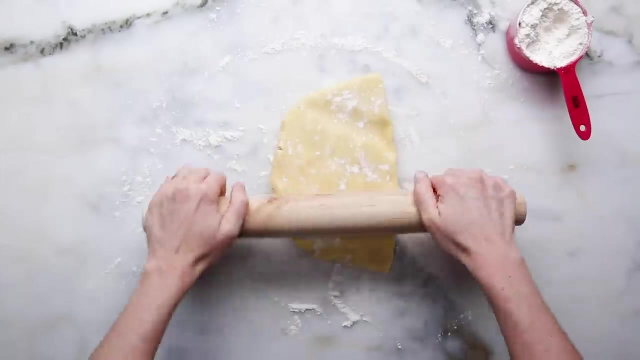 in culinary school. you really want an even quarter inch all throughout To get the most even thickness. you want to press down on your dough like this and it just kind of spreads it before you want to get into rolling. You want to press down on your dough like this and it just kind of 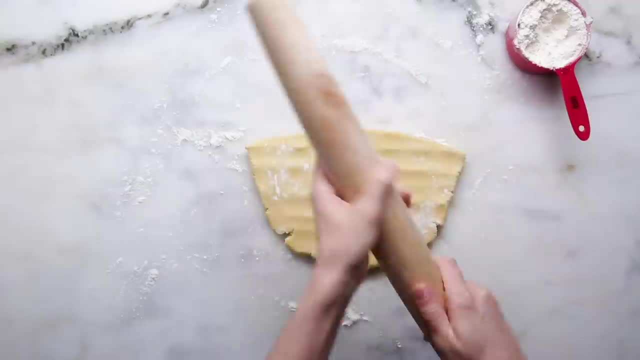 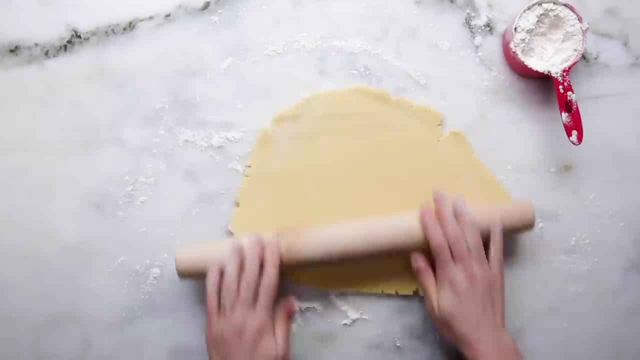 spreads it before you want to get into rolling Every so often. you want to do like a quarter turn, And that's going to help make sure that you have an even roll as well as to ensure that it's not sticking to the surface. This isn't like pie crust, where you really have to be careful about. 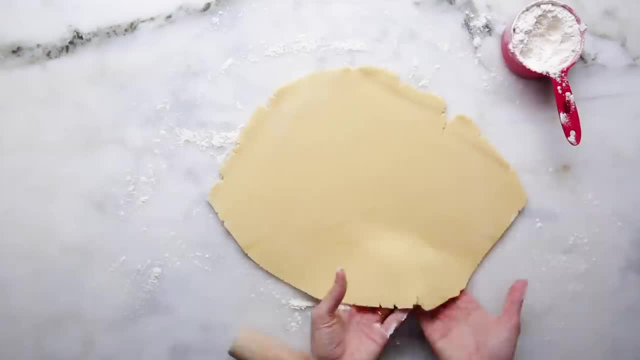 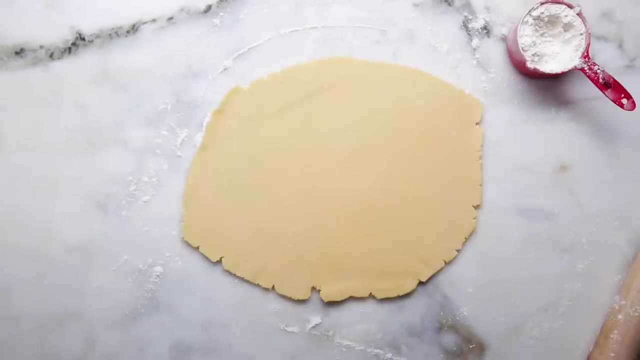 the shape that you're making or whatever. This is just kind of a free for all. So I'm to a good place. I'm not really sure how thick mine is, So how do I measure this? You could use a ruler, But 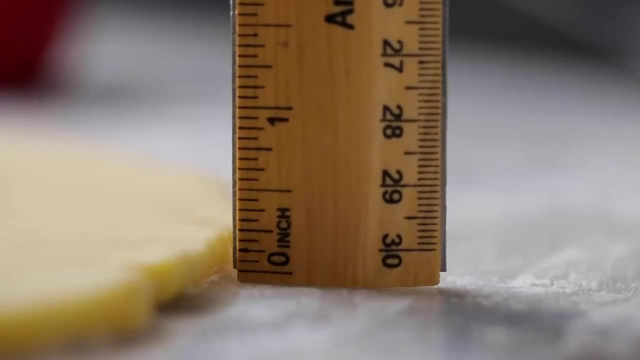 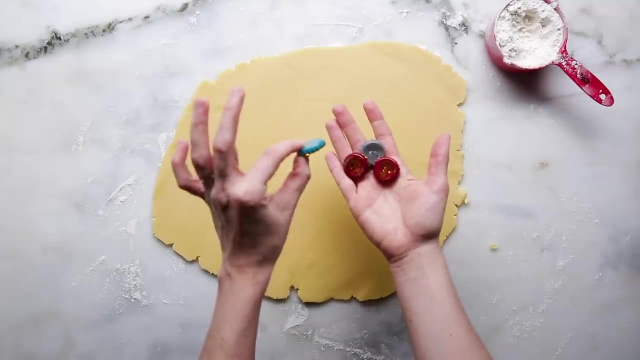 you know, what's so annoying about this ruler is like: why does the zero start so far up the ruler? It's not so annoying, But how else can you measure bottle caps? I was looking all over the kitchen for something else. that's a. 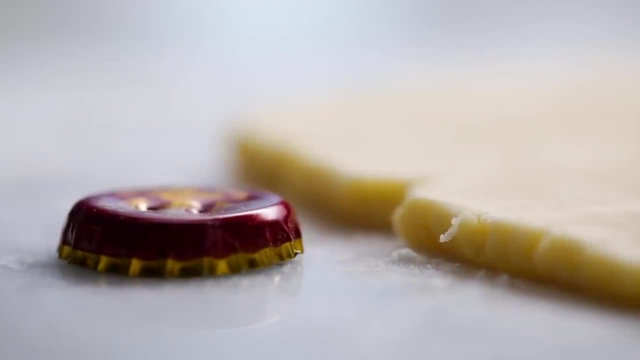 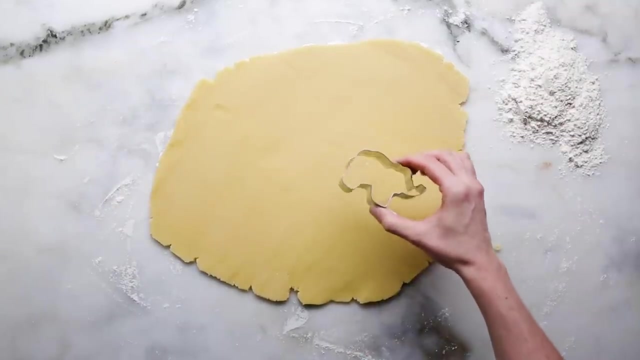 quarter inch. I like to lay these around the dough while I'm rolling out, just to make sure that all sides are that perfect quarter inch. The other thing, too, is pour out that extra bench flour, and that's what we're gonna use to flour our 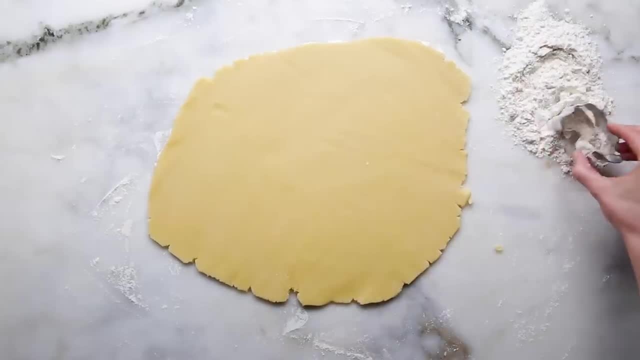 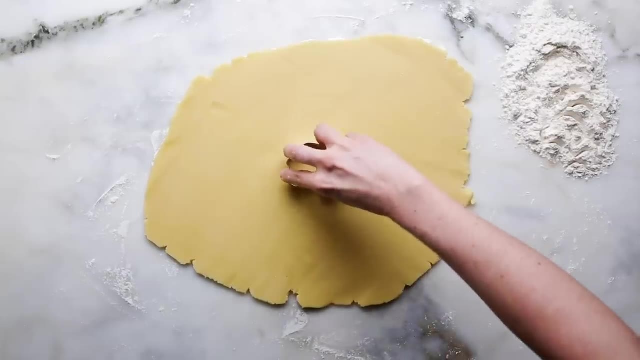 cutters, to make sure that the cutters aren't sticking too much to the dough. So dip the cutter all the way in flour, dip off the excess and then go ahead. And then just give it a little like zhuzh, a little shimmy, to make sure that you've 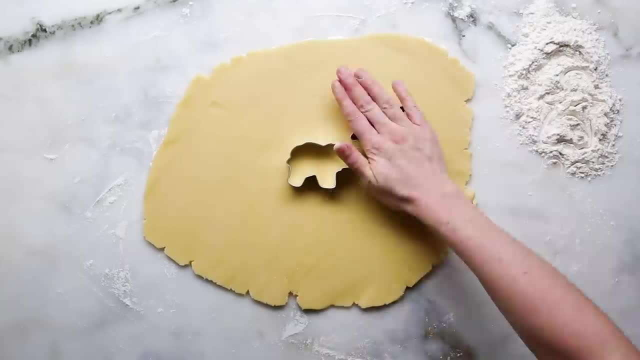 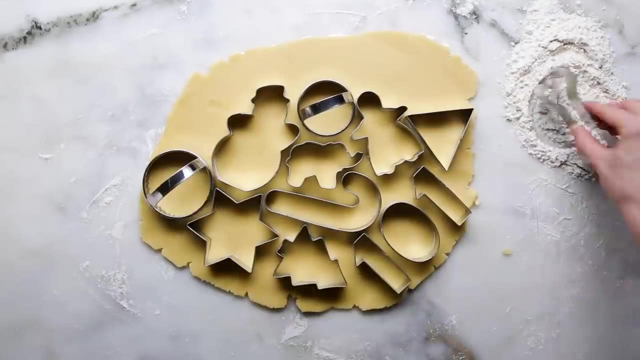 totally made contact with the surface on the bottom, And if you have enough cutters, what I like to do is go ahead and put all the cutters down and leave them, and that makes sure that nothing's pulling or tugging and you get a really 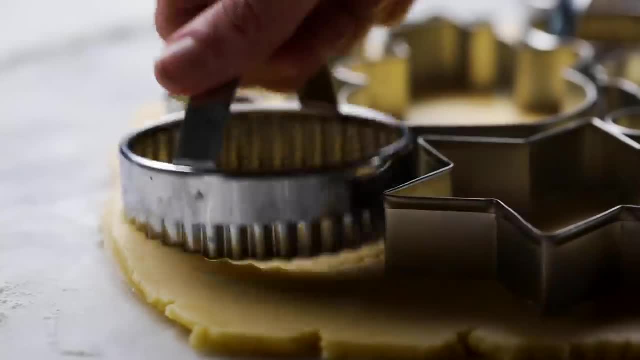 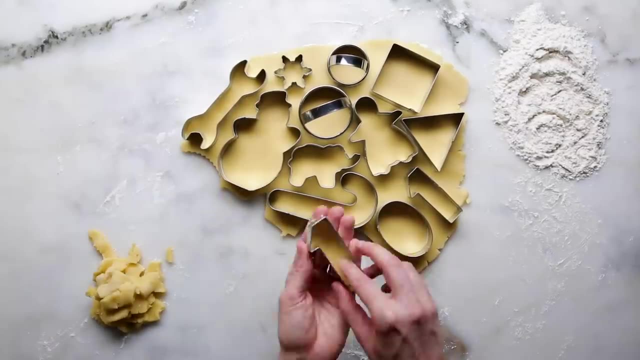 clean shape every time, And now you can start pulling them out. Sometimes the cookie comes with the cutter and sometimes it doesn't, So I like to kind of move around, pull off the excess, put it off to one side, save that dough. 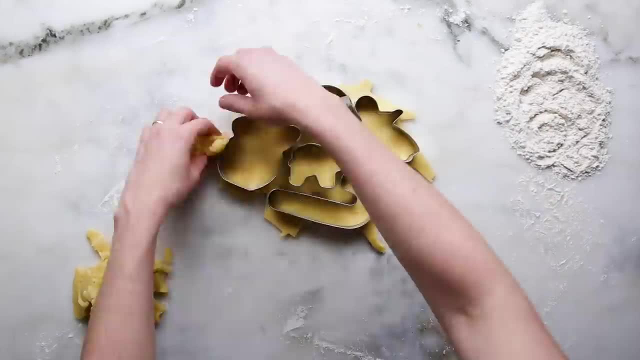 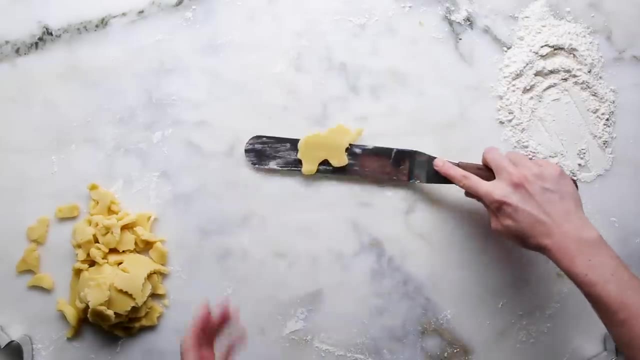 because you can use that again. Just be careful that you're not like pulling or tugging at everything because you really want the shape to be really clean And then you're good to go And then look at that So you can definitely reuse these scraps, What you. 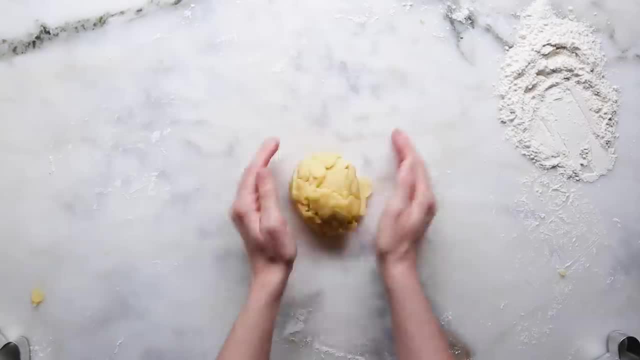 want to do is get them back into like a cohesive dough ball and then put them back in the fridge. They're really warm after all that rolling and working with them, So get the cold one out of the fridge and put that one back in there. 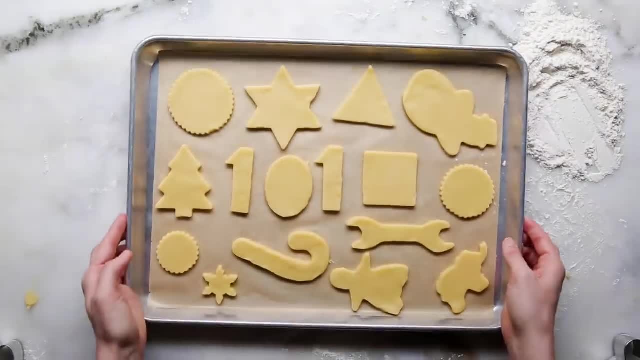 for another, like 20 minutes or so, so it can firm back up. And there we go. If you have some shapes that are smaller than the other ones, I would put those off to the side so that if you need to pull them early, you can, so that they don't. 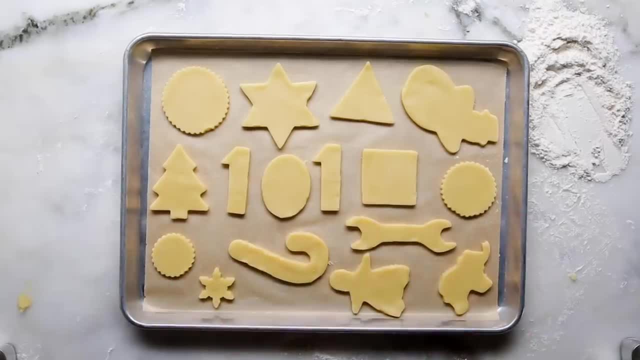 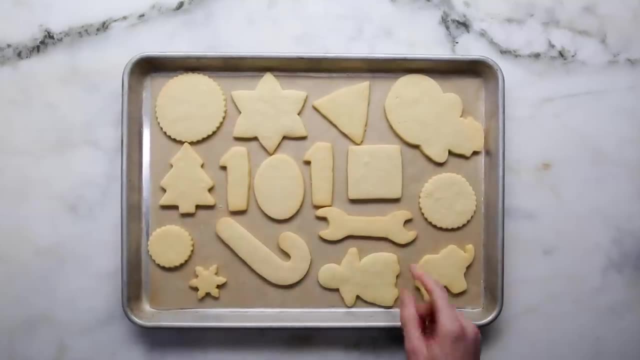 over bake. Okay, put these guys in the fridge. You put them in the oven now. they're going to spread way too much. They're not going to have a clean shape. They will come out super clean, super crisp. As you can tell, they're still very 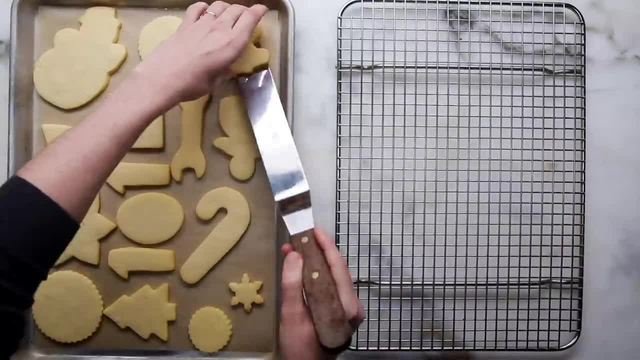 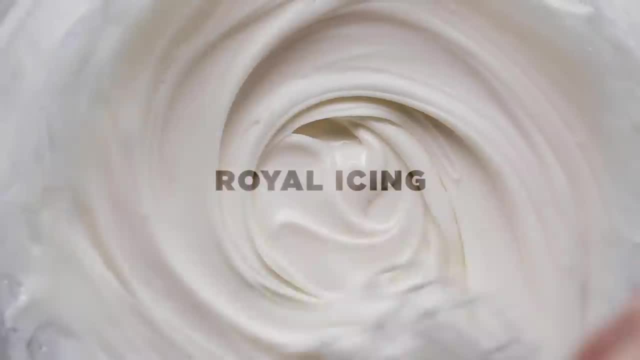 pale and they haven't spread that much. Yay, Go ahead and take them off and let them cool completely on a drying rack. Time to decorate. So we chose royal icing because it sets a little bit harder If you're gonna be really crazy with. 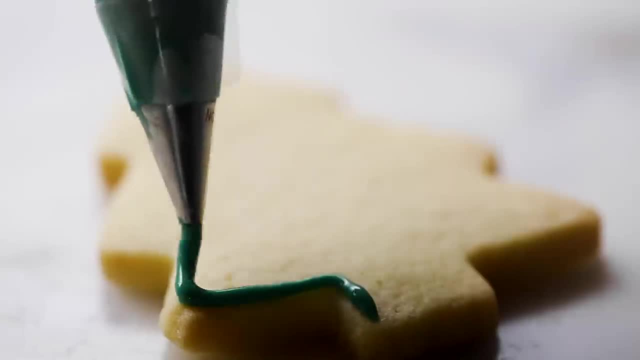 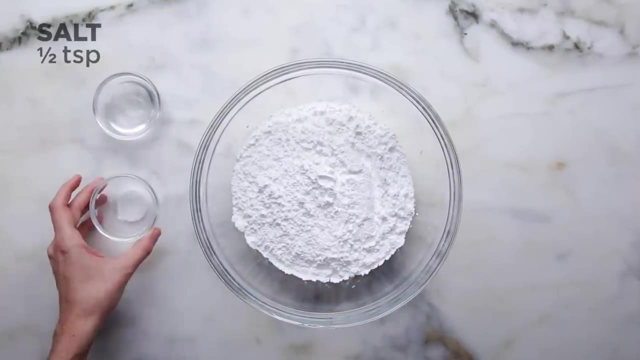 decorating royal icing is definitely the way to go. So, despite its royal name, royal icing is pretty simple, So all you really need is some sifted powder, sugar. You might need a little bit of water, A bit of salt- salt, an extract if you'd like it- and egg whites. The thing about this is that we 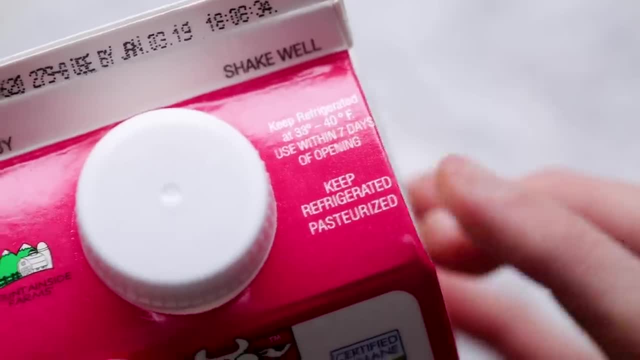 will be consuming this. so you really want to make sure that you're buying pasteurized egg whites so they're safe for everyone to enjoy. Or you can use meringue powder, which is an egg white substitute. We might need water. it kind. 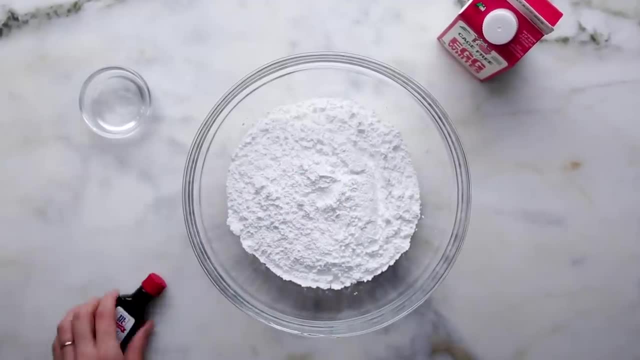 of depends on what we're going for, but first we're gonna add salt and a little bit of vanilla for flavor and we're gonna put this off to the side. So all the liquids we're gonna put on one side of the powdered sugar and I'll show you why. 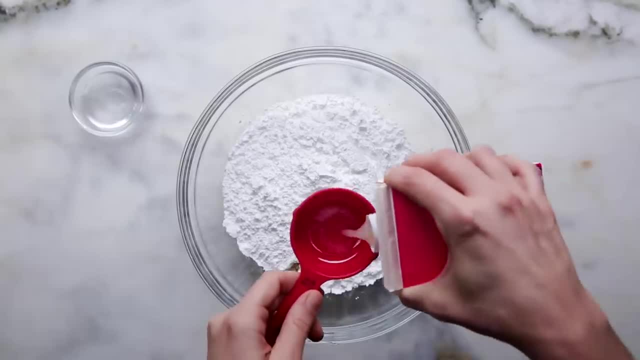 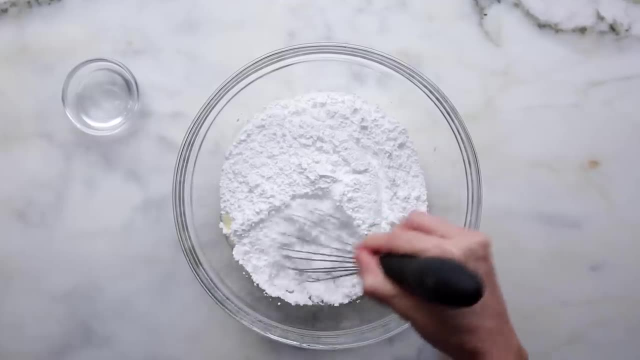 in a second, Make sure to shake those egg whites ahead of time and in they go Again, making sure that they're on one side of the bowl. And so now we're going to just work in that one part of the bowl and just slowly incorporate more of 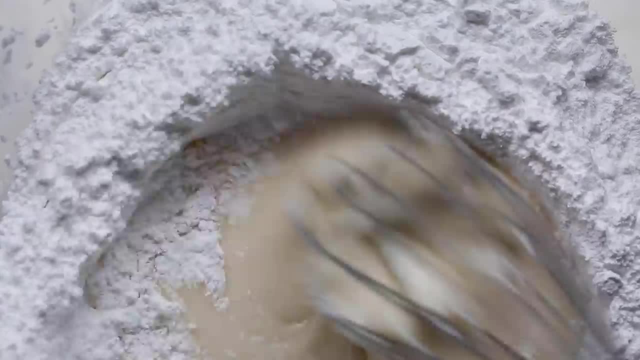 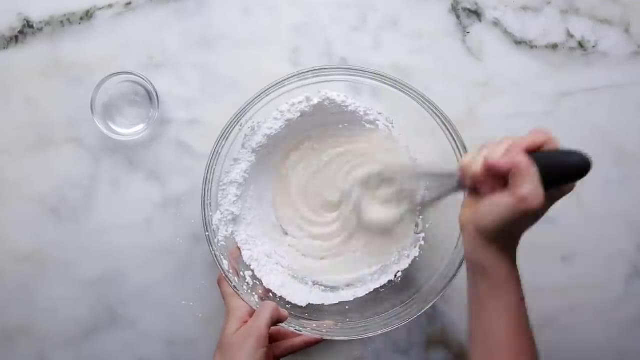 the powdered sugar as I go. That's gonna help make sure that I have a really smooth icing. If you're trying to incorporate all of that powdered sugar at once, it's just like a little bit harder to work with and also you probably will get some lumps. Royal icing is all about consistency, so depending on 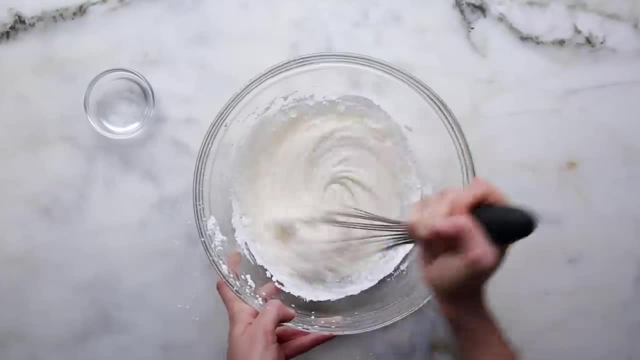 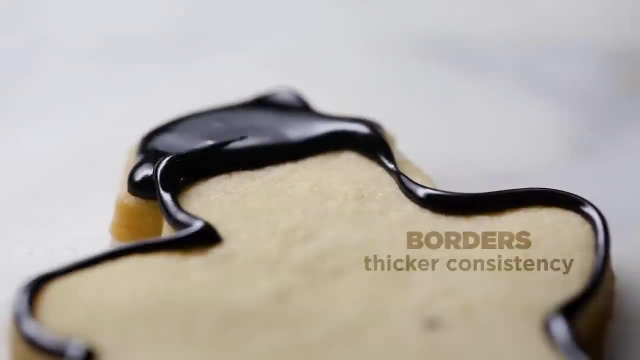 how you want to decorate yours. there's kind of like two consistencies that you're going for. There's a thicker consistency for more of like lining things out or like borders of things, and there's a flood which is gonna be just a thinned out. 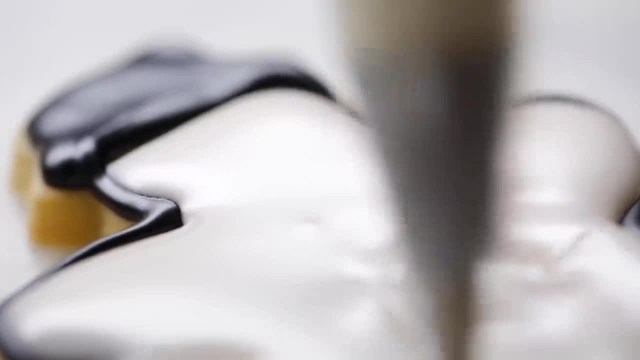 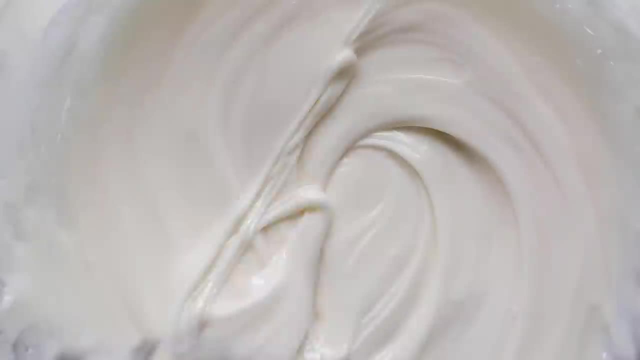 version, And that water is gonna come in handy when we're looking for that flood consistency. So we're starting here with a thicker royal icing. We're also gonna add coloring to this, which will thin it out a little bit too. So air on the side. 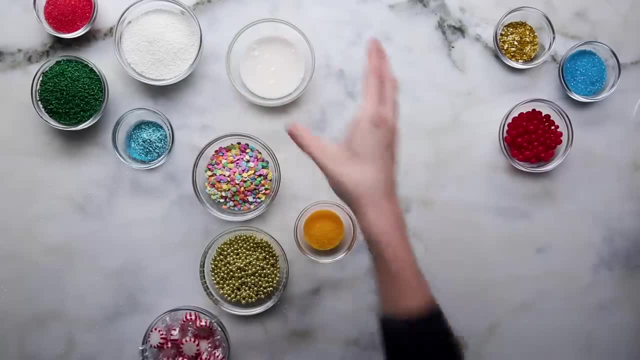 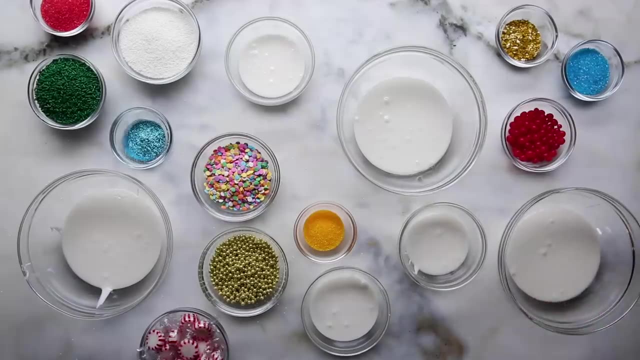 of thicker when you're getting started, So we're gonna separate the icing into a few different bowls. If you're gonna be doing a lot of decorating or using a lot of different colors, it's probably worth it to double or even triple this recipe. Go ahead and put in your gel food colorings to get really, really. 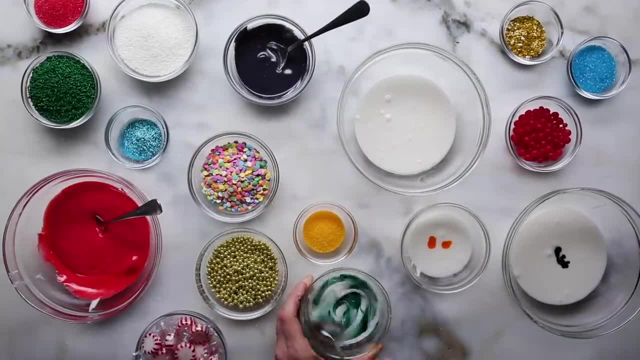 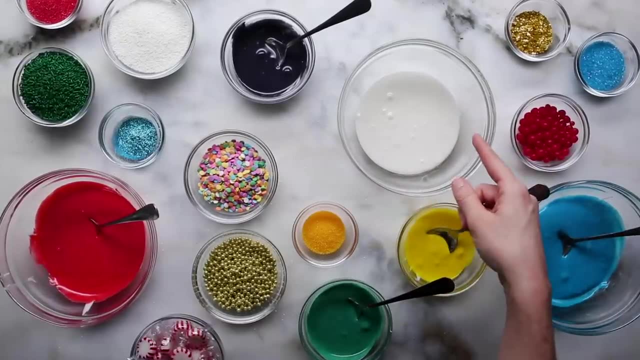 bright colors. The thing that's cool about royal icing is it sets right, So it'll set kind of hard Even in this time. while we're trying to get everything set up, you can already see a little bit this kind of skin that forms on top. So 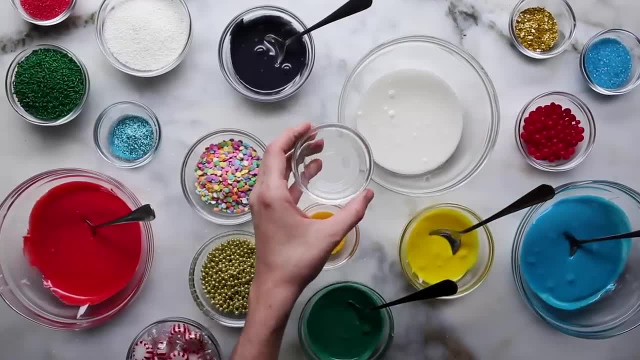 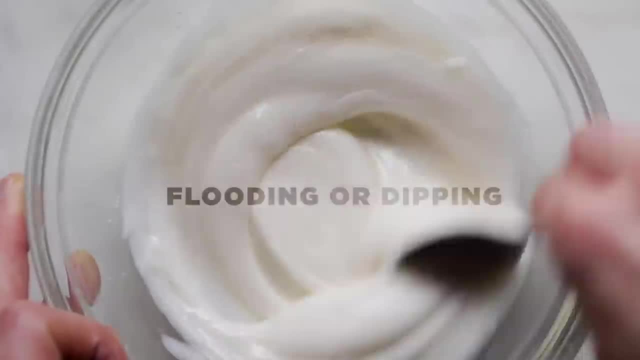 you do want to work a little bit quickly with royal icing, or else cover it with cling film And then just to fix it, just add a little bit of water and stir. So now we can do one of two things with this flood: consistency: Flooding or dipping. 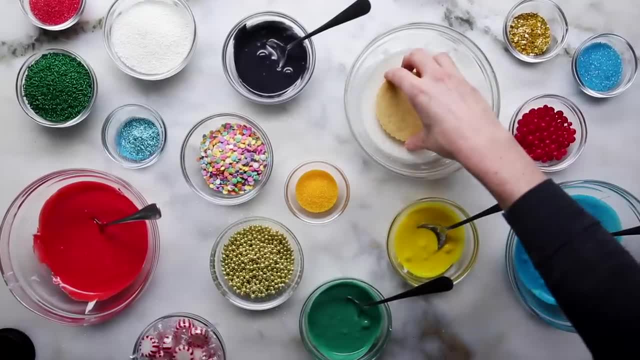 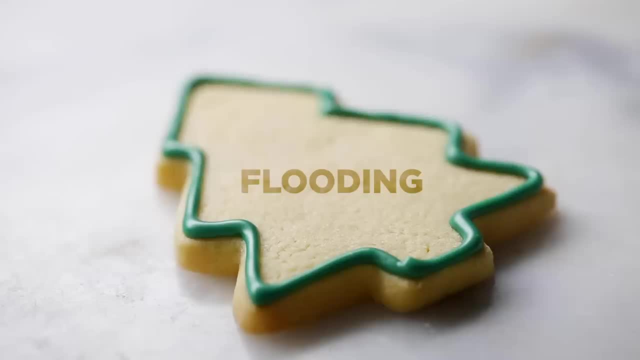 And then you want to let that kind of harden for a little bit before you go to the next step. So go ahead and put the cookie, dip it in the icing, make sure it's really well coated, Knock off any excess, and then it's going to kind of 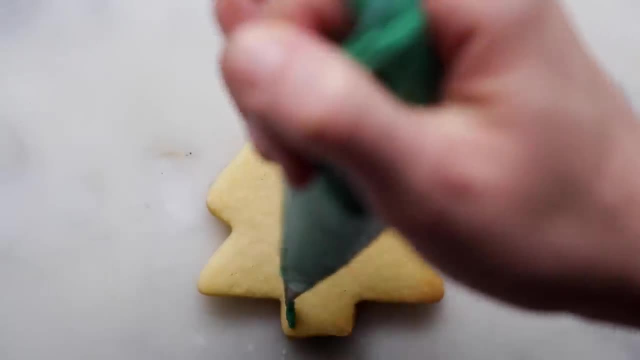 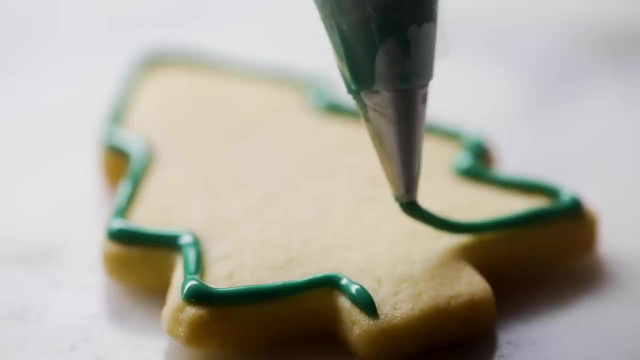 settle into the cookie and be a really smooth and even shape And then to flood what you got to do. you want like a thicker frosting in a piping bag, and then go ahead and just trace the outside with whatever color that you're doing. 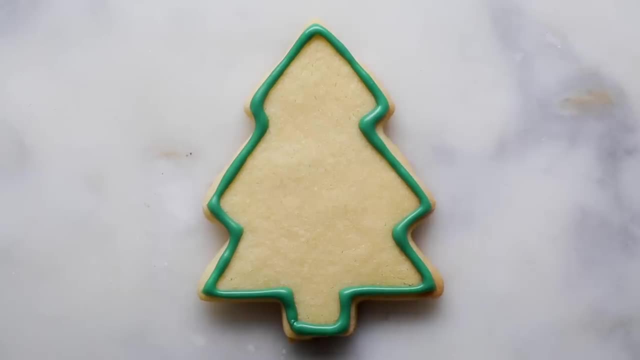 And then you want to let this harden for a little bit before you go to the next step. But once it is hard, all you need to do is take that thinned out icing and spoon it in, like I'm doing, or you can also put it in a piping bag and pipe it. 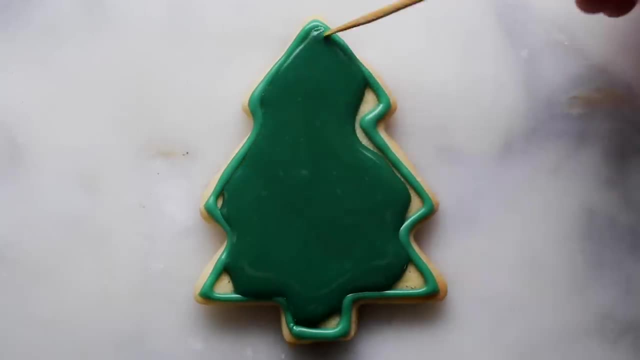 in and then use the toothpick to spread it out evenly. That bit that you piped in the beginning is dried, so it kind of acts like a wall or a border to ensure that all of that icing is staying inside. If you're gonna put sprinkles on it, go. 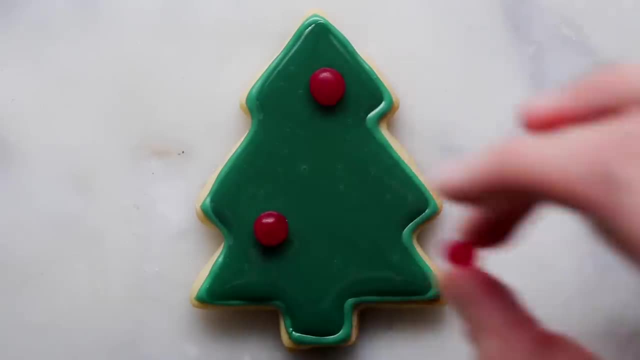 ahead and put the sprinkles on when it's wet. but if you want to decorate over that, go ahead and let that set for a good like 10-15 minutes or so and then you can continue decorating on top of it. So it kind of depends what look you're. 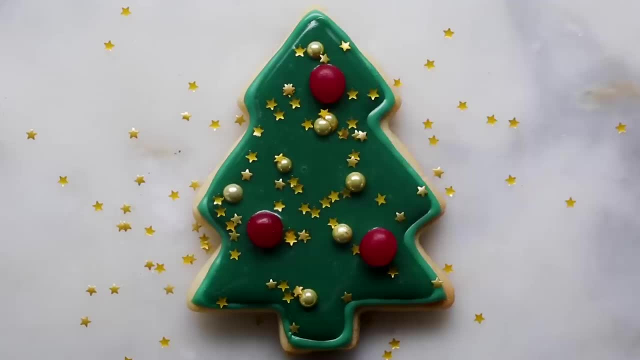 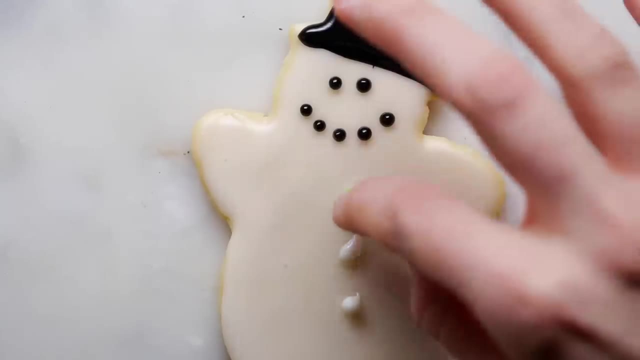 going for And, as you can see, like these dots are kind of settling on top of it and not really falling into that flood, And then if you want to decorate any more or put any other like toppings on top of it, you're gonna have to layer. 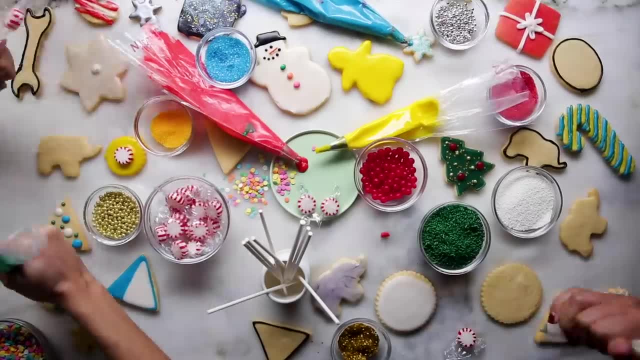 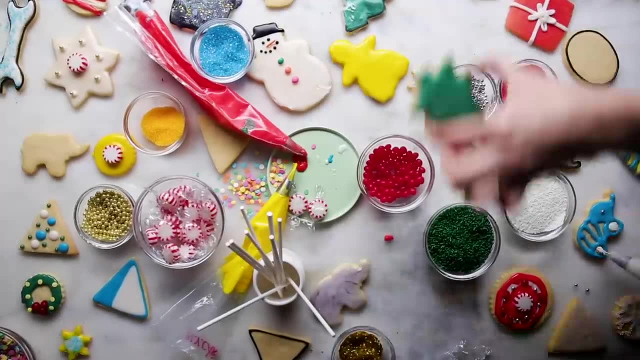 more icing on just to make sure that they stick. There's like something magical about this Baking cookies. it's kind of like what gets you ready for the holidays, right? Like you know, it's the holiday season when it's time to bake the sugar cookies and it's time to decorate them, and you know people really.